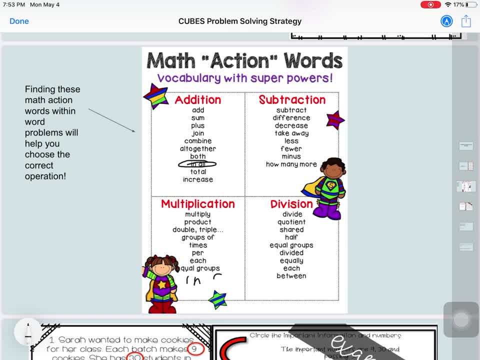 you clues on whether or not you're going to be able to solve the problem and they give have to add. sometimes you might even see in all when you have to multiply. if you see how many more, that's a clue. you need to subtract. if you say, if you see. 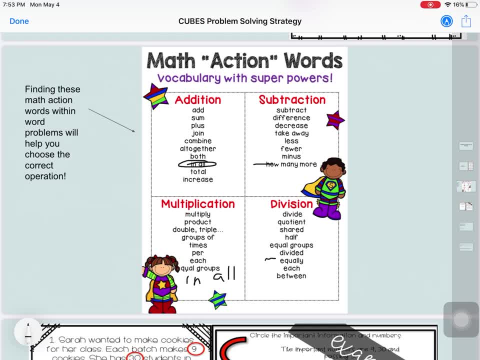 something like it's: all these are divided equally. that is a clue you need to divide, so this is a great tool for you, this sheet. you could always go back to this part in the presentation and and take a screenshot of this. this is a really great tool for you, a great resource when you're solving word. 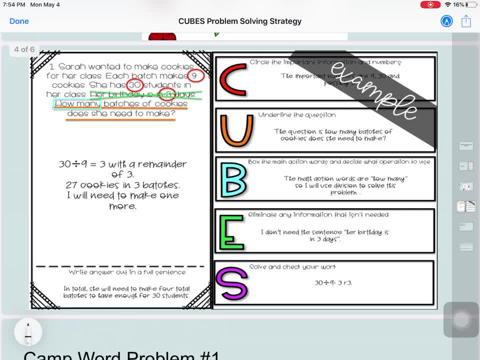 problems, which can be tricky, okay, so let me show you an example. Sarah wanted to make cookies for her class. each batch makes nine cookies. she has 30 students in her class. her birthday is in three days. how many batches of cookies does she need to make? 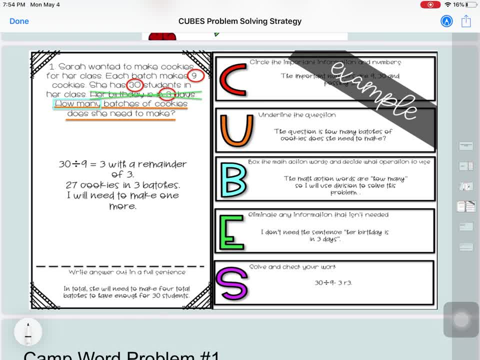 so the first step is to see circle the important information in numbers. so we have 30, 9 & 3 circle you underline the question. the question is at the end. typically it says how many batches of cookies does she need to make. so that's underlined in orange B. you can box the math action words and decide. 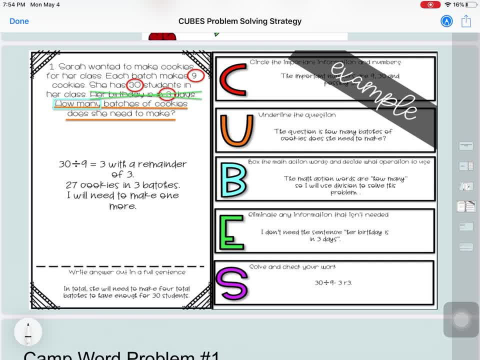 what operation to use. so the math action words are how many here, and we're talking about batches or groups of cookies. so in this case, how many? is signaling a division problem? E eliminate any information that isn't needed. where it says her birthday is in three days, that's crossed out because we 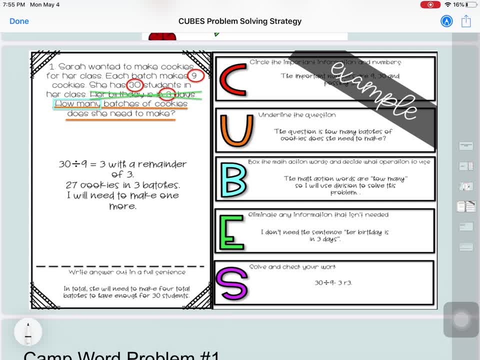 can eliminate that. we don't need that information to solve the problem and then solve and check your work. so, 30 students in class. she wants to know how many batches she needs to make. every batch has nine cookies, so we know we need to divide 30, divided by 9 and it would be 3 remainder. 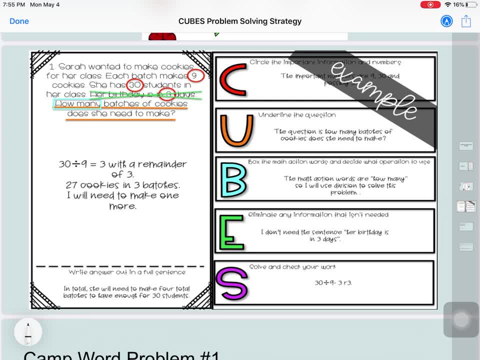 3, because if you, if you skip, count by 9, how many times does it go into 30, 9, 18, 27, Oh, 36 would be too much. so we have to stick with three times and we would get a remainder of three. so you wouldn't just stop with three batches and have 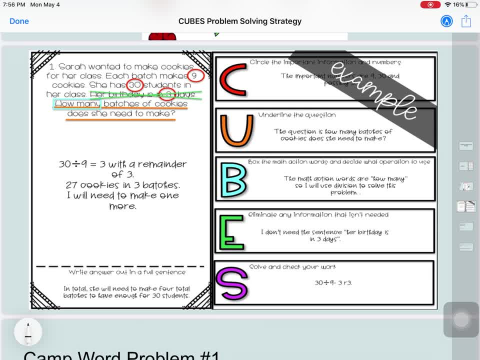 three remaining cookies and not enough for all the kids, you have to cook another batch so everyone gets enough, okay? so that's an example of how we use the strategy. with a word problem, let's try it out with your camp problems for this week. so now we'll. 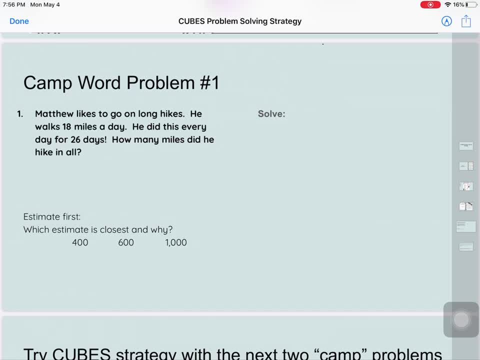 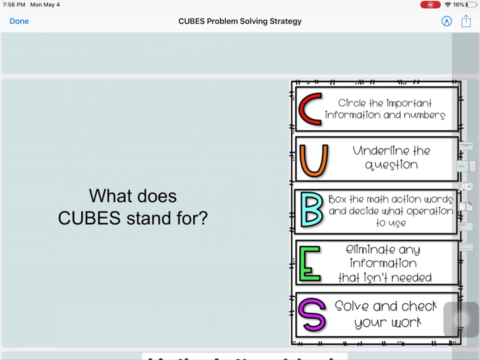 go to our camp, problem number one. so this is on your learning plan for today. Matthew likes to go on long hikes. he walks 18 miles a day. he did this every day for 26 days. how many miles did he hike in all? so I'm going to go back to the steps again. first I need to circle the important. 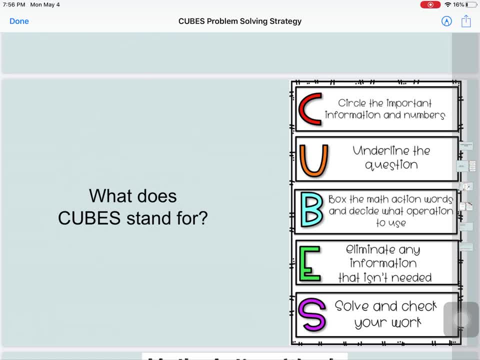 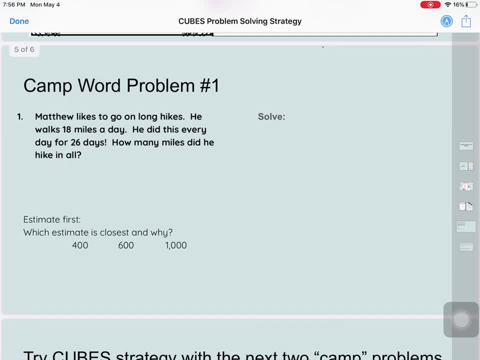 information number in numbers you underline the question. I'm going to do those two steps: first, circle and underline the question. okay, I have to circle the important information 18 miles a day and then for 26 days. while that's intense, that's a lot of hiking. then I know I need to underline the question. how did 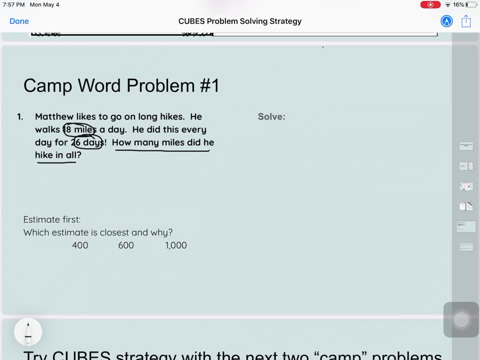 he hike. then you see B, b is my next step. box the math actionworm words and decide what operation to use. I'm going to go back into that problem. Are there any clue words? How many miles did he hike in all? Oh, I'm going to box in all. That could either mean to: 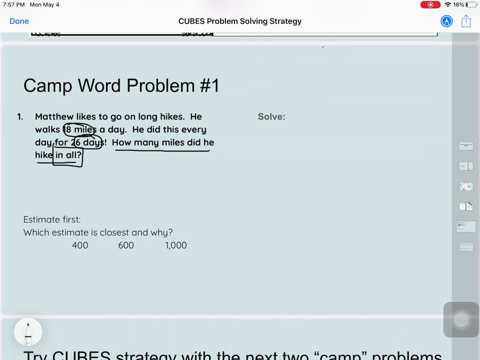 add or multiply. Since we're talking about 18 miles a day for 26 days, I'm not going to add 18 26 times. That doesn't make sense. I'm going to multiply. That would be more efficient. So it's a. 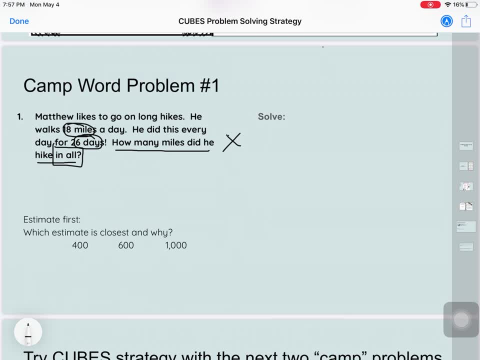 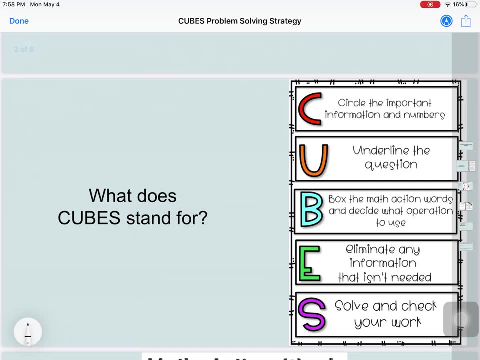 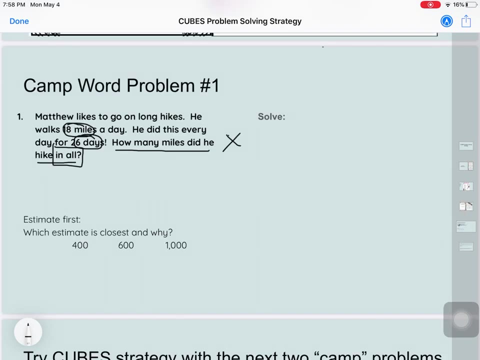 multiplication problem. I'm just going to write that to the side, So to remind myself. I'm going to multiply And E- eliminate information we don't need. And then S is solve and check your work. Okay, so I'm going to go back, Eliminate. Is there something I don't really need to know? Well, I. 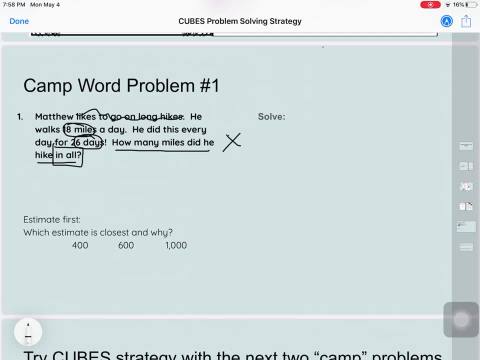 don't really need to know that he likes going on hikes. I don't really need that. If it helps you, you can cross things out. So you're really just focused on what you need for solving. Okay, so, in order to solve, they're asking us to estimate first And remember when we're 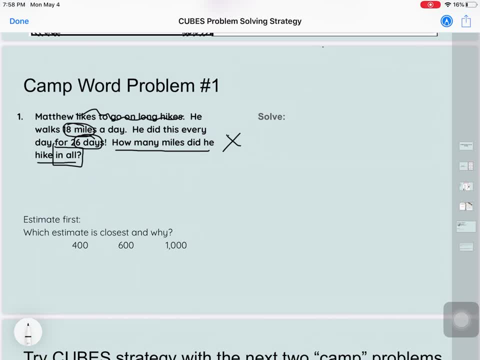 estimating. we're kind of we're either rounding numbers or changing them into nice numbers so we can just get a quick estimate. Estimates are really great because when we solve we can check with our estimate to see if our answer makes sense. So 18, I could just round that up to 20.. 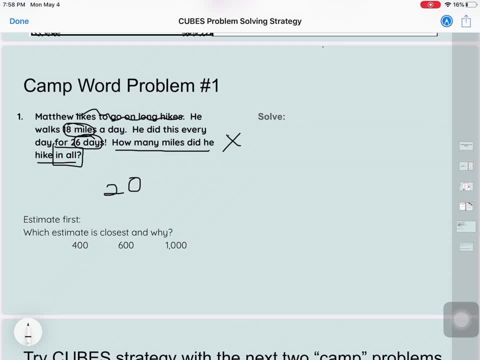 And then 26.. 26 is really close to 25, which is a great number to work with because you can think of quarters And I have a multiple of 10 here. I could just look at my basic fact of two and then 25.. And 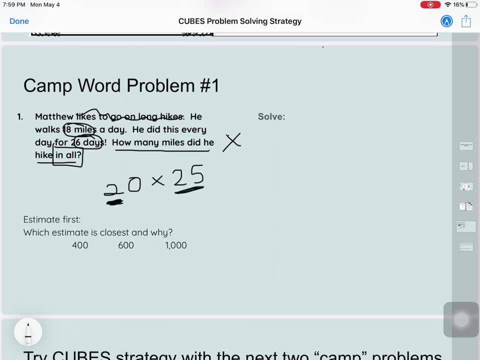 just ignore the zero right now. What's two times 25?? Right, it's 50.. And then I could write in the zero: So then 25 times 20, if 25 times two is 50, then 25 times 20 is 500.. Which estimate? 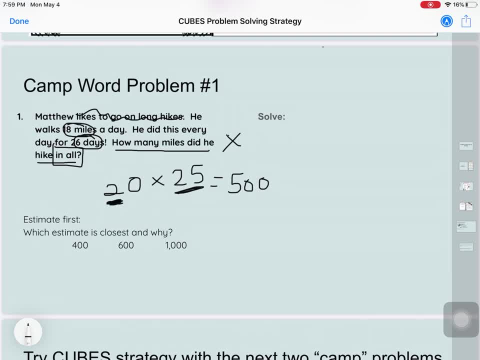 is closest. Well, it's not on our choices: 400, 600, 1000.. I'm just going, even though it's not here, I'm just going to write in my estimate because I think I got very close. I didn't change. 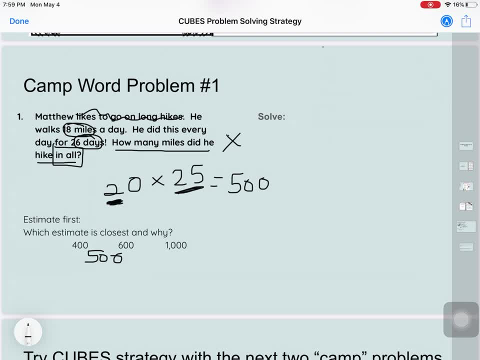 the numbers very much, from 18 to 26.. So I'm going to say 500 because my numbers are very close. So I think actually 500 is a better estimate. I know it's not an option, but let's go with that Are very close. 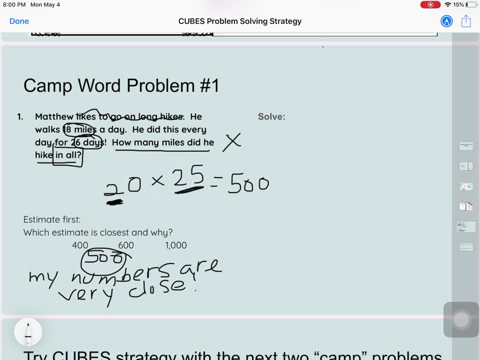 Okay, now I can solve. So it's been a while. but we've been familiar with solving two times 200.. by two digit numbers, by making area bottles, So we have 26 days and 18 miles a day. So I'm going. 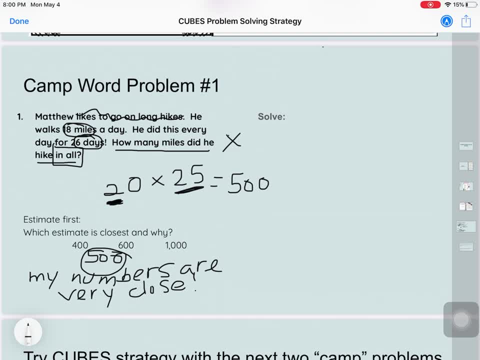 to draw 26 on top. I'm going to draw kind of a longer line to represent 20.. So we have 20, I'm going to break that up to 20 and 6.. Then I'm going to take 18 and make a box here. 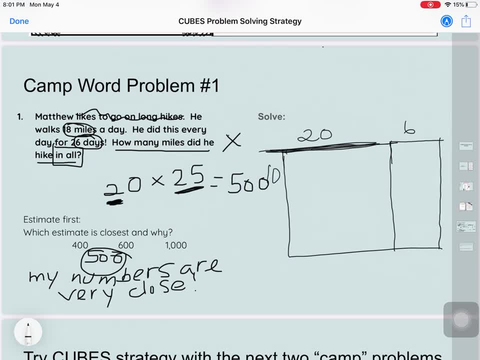 And 18,. I'm going to break that up into 10 with a slightly longer line. Let's say: let's say 8 is right here. So 10, 10 and 8,, 20 and 6.. So now I'm going to multiply. 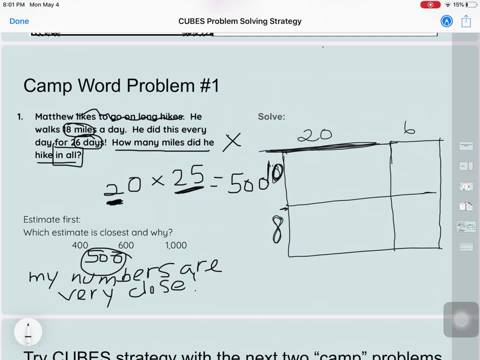 the rows and columns here and I'm going to put my answers in the middle. We're going to add these all up, So we're breaking this into partial products. We're finding partial answers and then we'll add it all up. So 10 times 20, I know is 200.. You could just look at your. 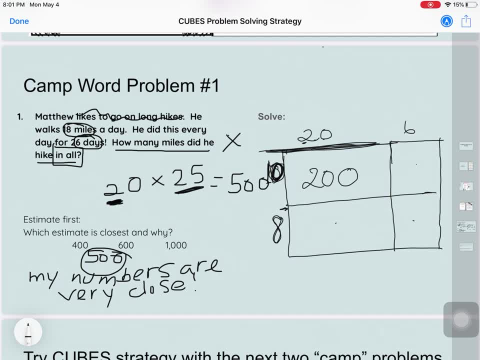 basic fact: 1 times 2 is 2.. Then add the zeros: 8 times 20,, 8 times 2 is 16.. And then we add the zero 10 times 6,, 60.. 8 times 6, 48. Now I'm ready to add this all up. I'm going to add up my larger. 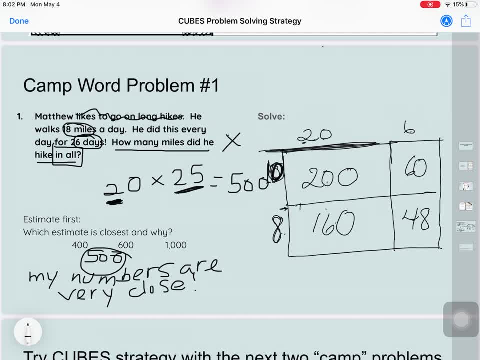 numbers. first, 20 plus 160.. I could just go down, It's 360.. Plus what would this be? 60 plus 48. Well, I know, 60 plus 40 is 100. And then I just add the 8. So 108.. Add those up: 468.. So you can kind of see from my estimate it's pretty close. 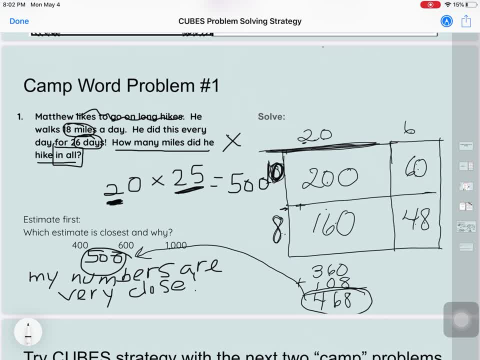 to 500.. So there we go. We just used the cube strategy to help us determine which operation to use, to help us determine the important information we need to solve, And we use an estimate to help us see if our answer made sense. So try this cube strategy.